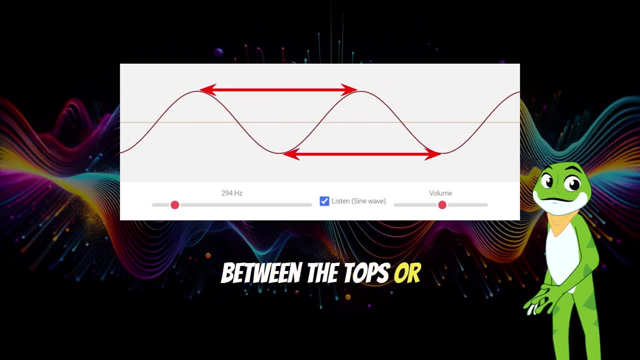 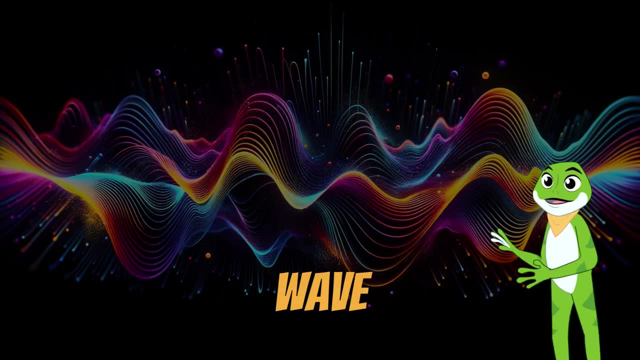 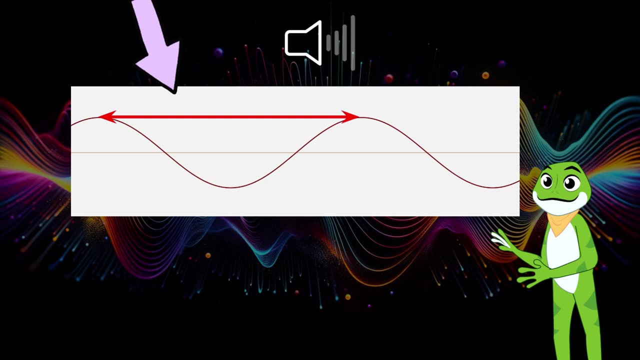 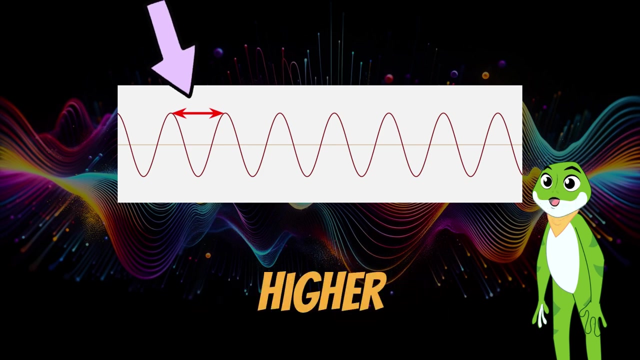 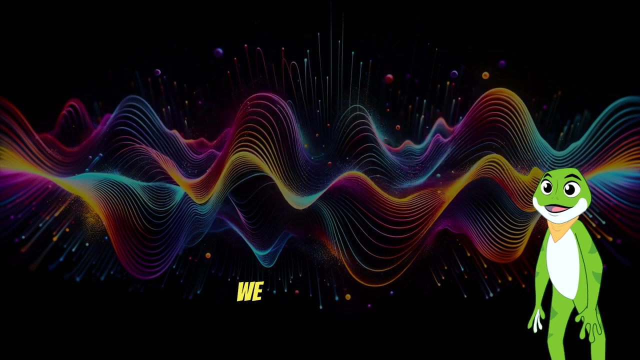 And the horizontal distance between the tops or bottoms of the waves is called the wavelength. When a wave has long wavelengths, it means that it has a low frequency. If a wave has short wavelengths, it has a higher frequency. We might say this wave has a deep sound because it has large wavelengths. and if we shorten, 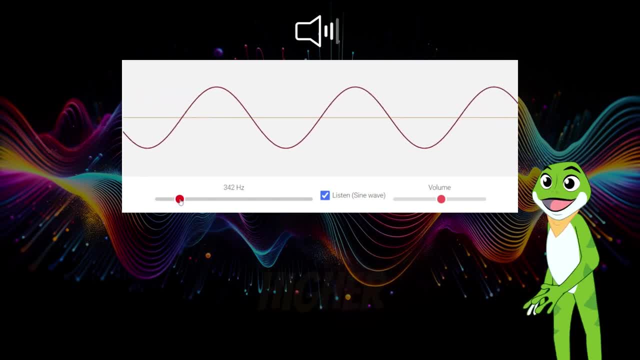 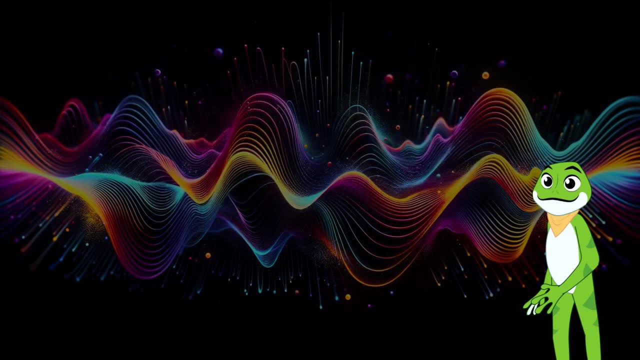 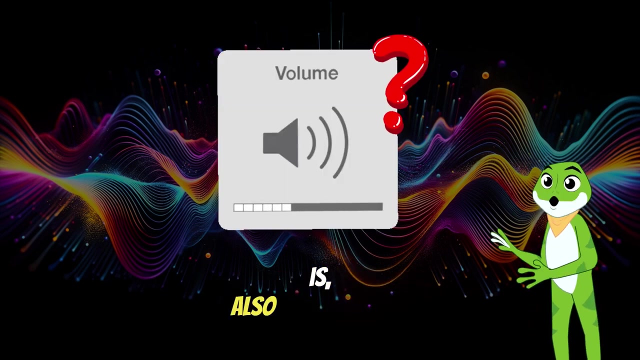 the wavelengths, we get a higher-pitched sound. So sound waves with shorter wavelengths have a higher frequency. But if wavelength determines the pitch of the sound, what determines how loud the sound is also known as the volume. Well, that's where amplitude comes in. 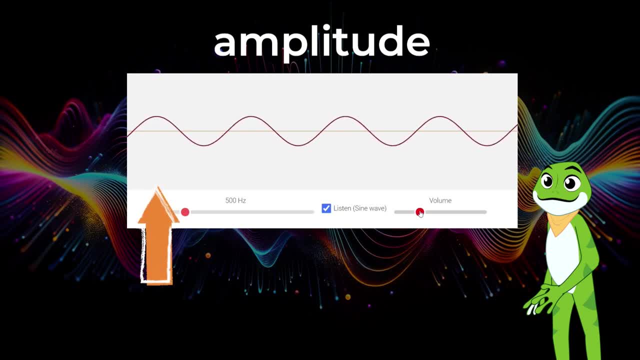 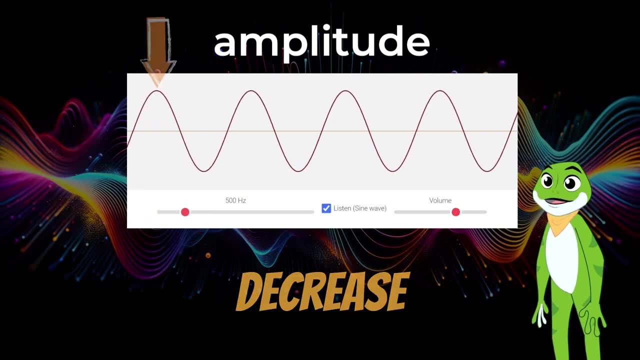 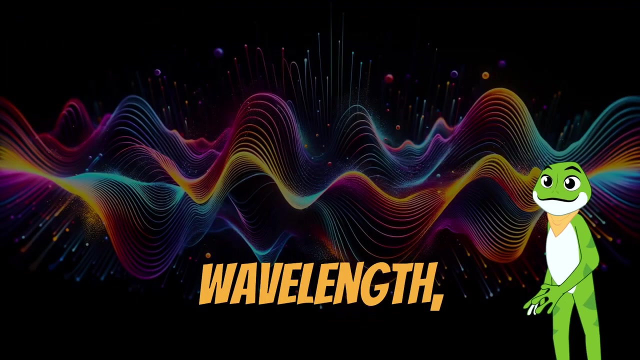 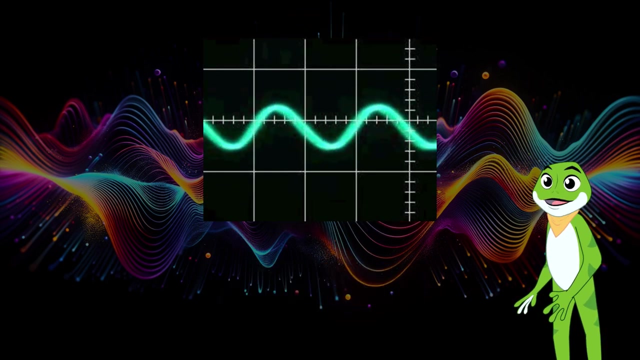 If we increase the amplitude, we get a louder sound, And if we decrease the amplitude, we get a more quiet sound. Now that we know about amplitude and wavelength, let's listen to a few sounds and try to determine what their sound wave looks like, based on how they sound. 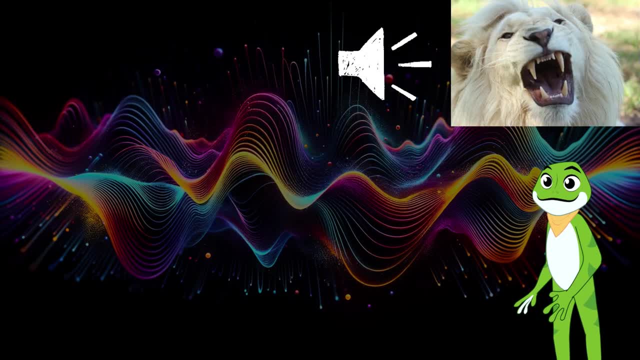 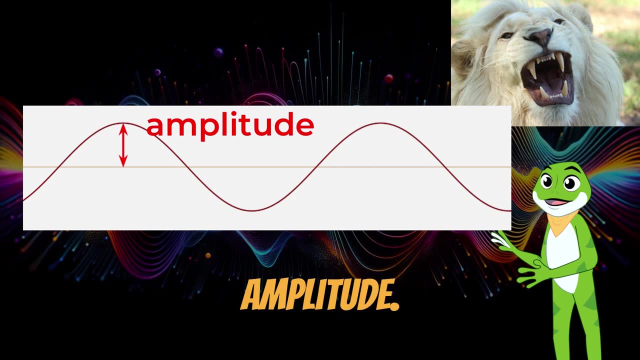 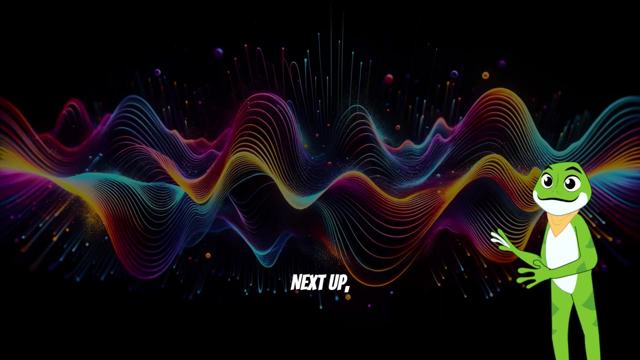 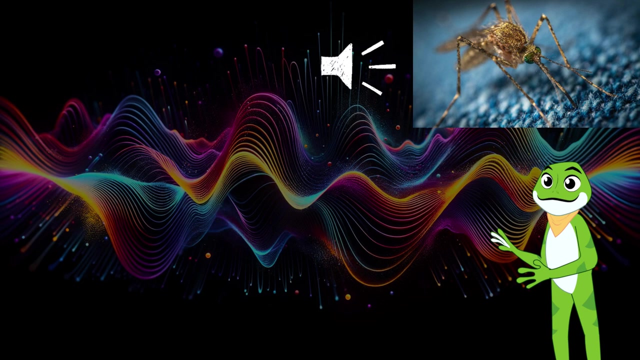 First up, a lion's roar. This sound is very loud, so it has a high amplitude, And it has a pretty deep sound, so it has a long wavelength, also known as a low frequency. Next up, an annoying mosquito flying around nearby. 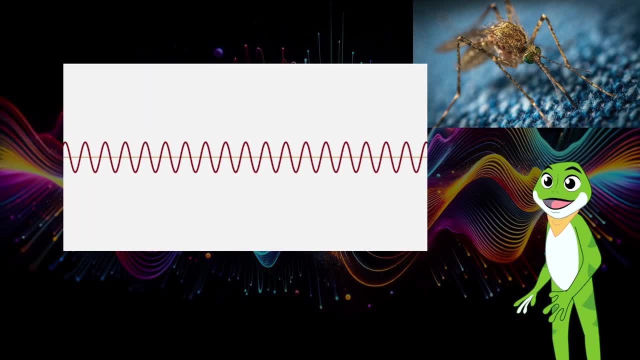 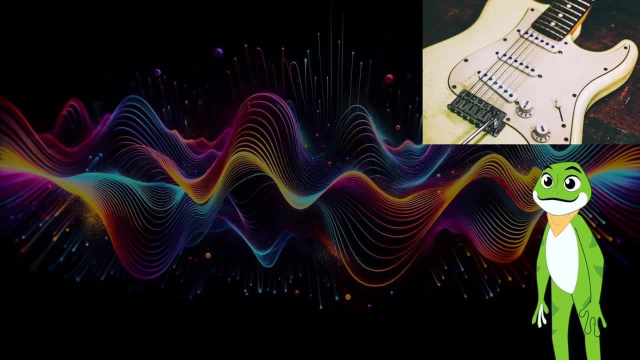 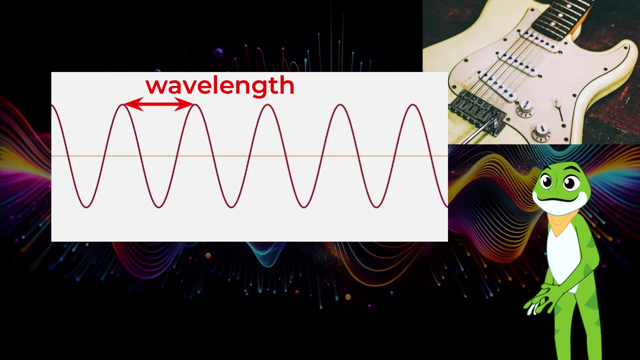 It is a very high-pitched sound, so it has a very short wavelength, also known as a high frequency, and it is pretty quiet, so it has a shorter amplitude. Finally, let's listen to this electric guitar. It has a high frequency, which means it has smaller wavelengths.